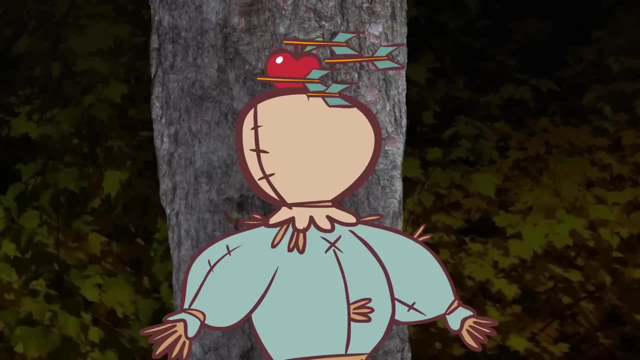 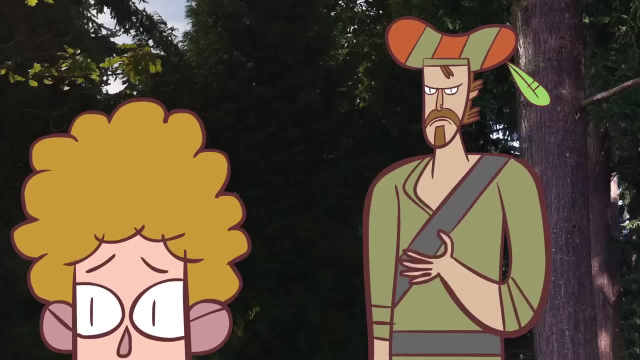 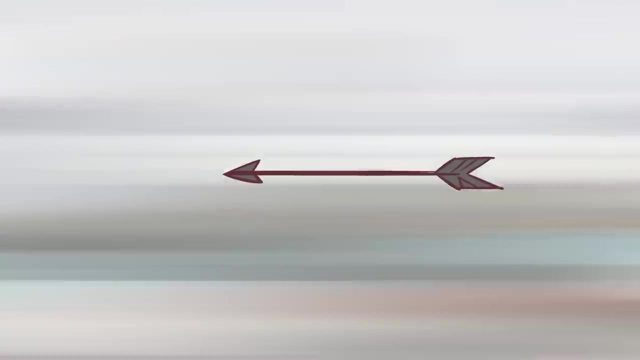 but in a random pattern. Occasionally he hits the apple, but with the wobble there is no guarantee of a bullseye. He must settle his nervous hand and restore the certainty in his aim to save his son. At the heart of these variations are two terms often used interchangeably. 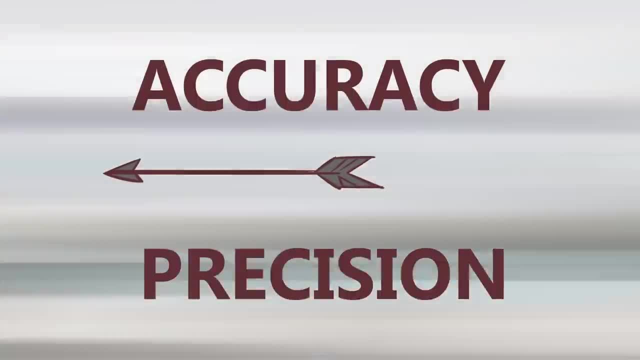 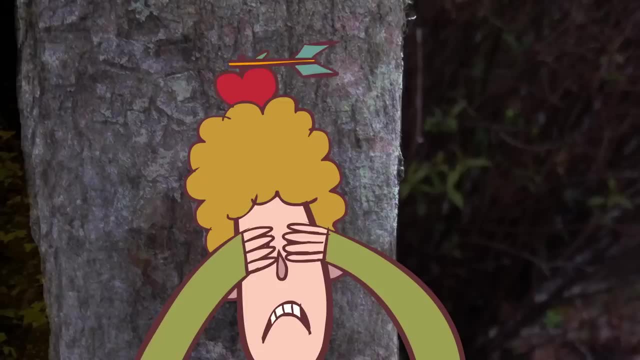 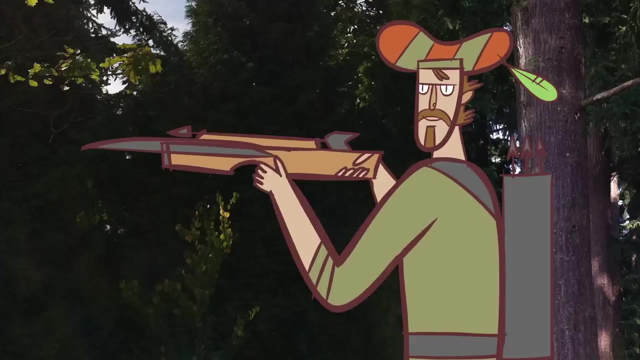 accuracy and precision. The distinction between the two is actually critical for many scientists. In fact, accuracy is the key to scientific endeavors. Accuracy involves how close you come to the correct result. Your accuracy improves with tools that are calibrated correctly and that you're well trained on. 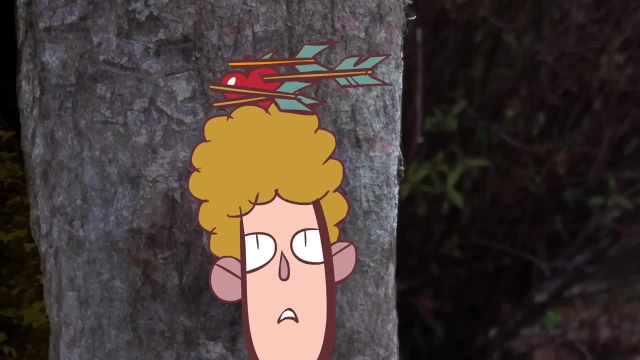 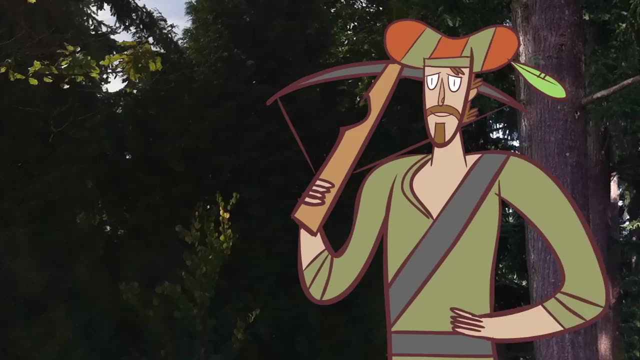 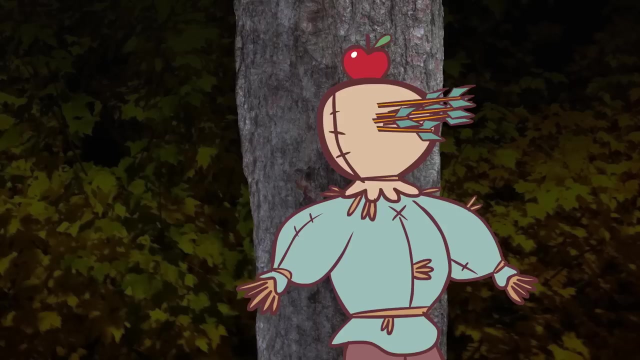 Precision, on the other hand, is how consistently you can get that result using the same method. Your precision improves with more finely incremented tools that require less estimation. The story of the stolen crossbow was one of precision without accuracy. William got the same wrong result each time he fired. 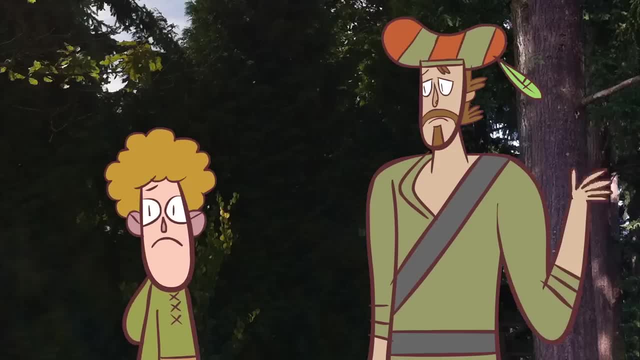 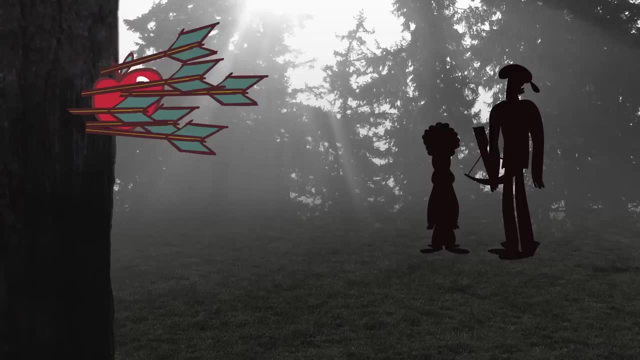 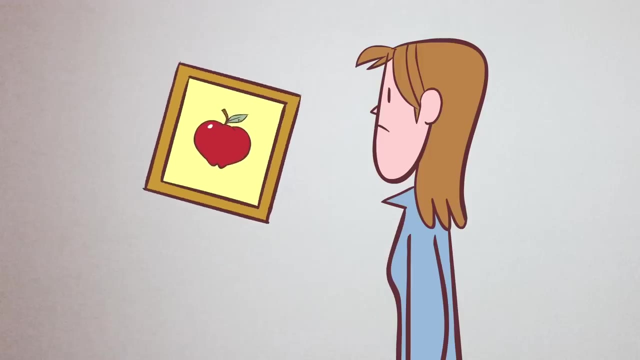 The variation with the shaky hand was one of accuracy without precision. William's bolts clustered around the correct result, but without certainty of a bullseye for any given shot. You can probably get away with low accuracy or low precision in everyday tasks, but engineers and researchers often require accuracy. 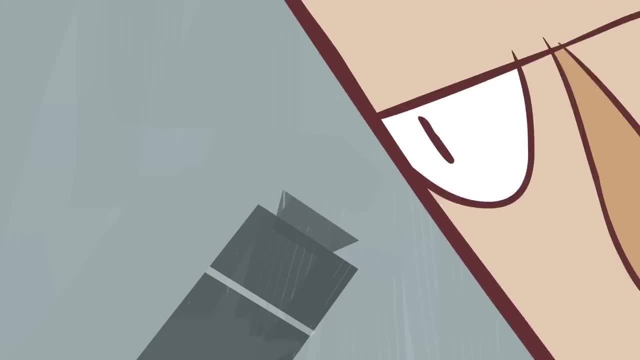 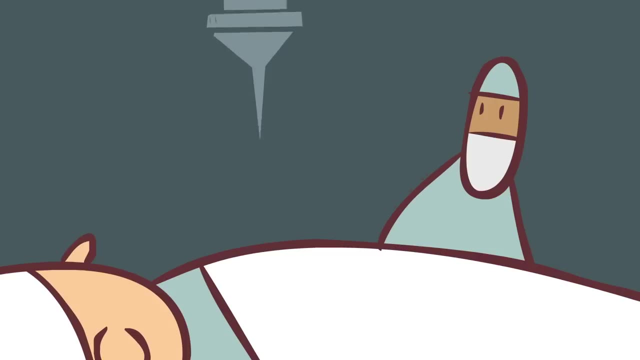 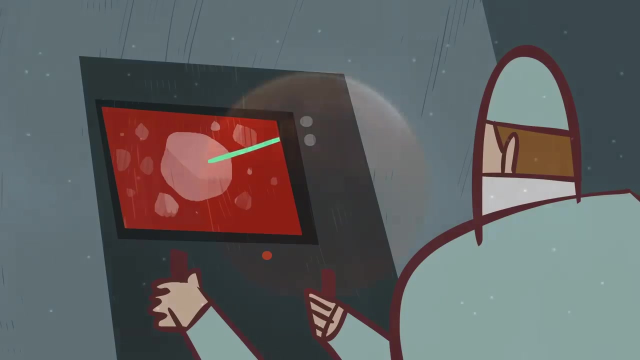 on microscopic levels with a high certainty of being right every time. Factories and labs increase precision through better equipment and more detailed procedures. These improvements can be expensive, so managers must decide what the acceptable uncertainty for each project is. However, investments in precision can take us beyond what was previously possible. 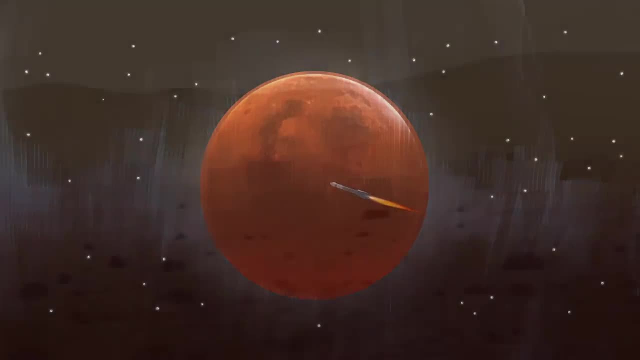 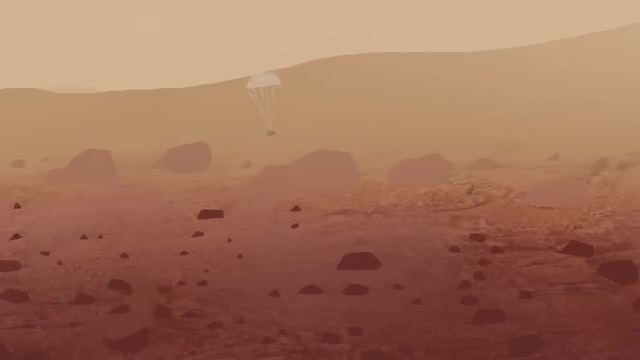 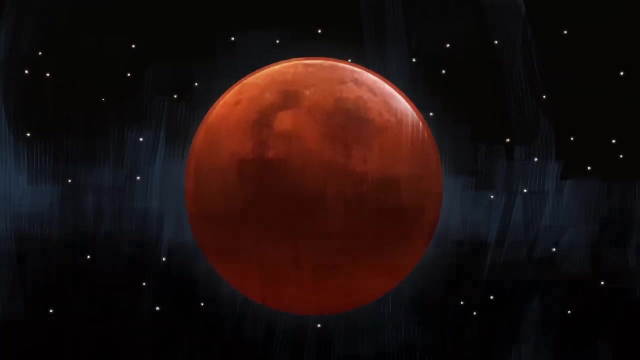 even as far as Mars. It may surprise you that NASA does not know exactly where their probes are going to touch down on another planet. Predicting where they will land requires extensive calculations, fed by measurements that don't always have a precise answer. How does the Martian atmosphere's density change at different elevations? 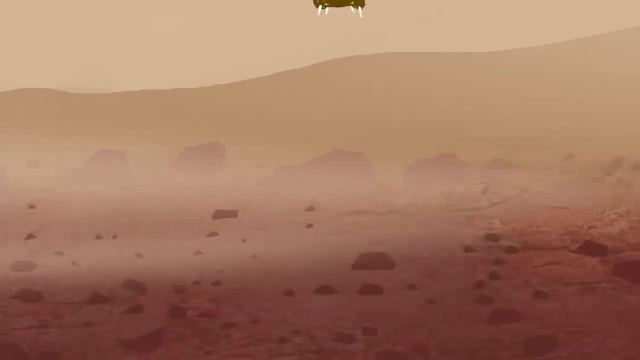 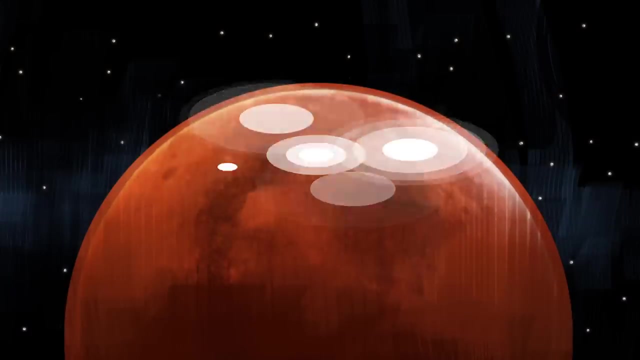 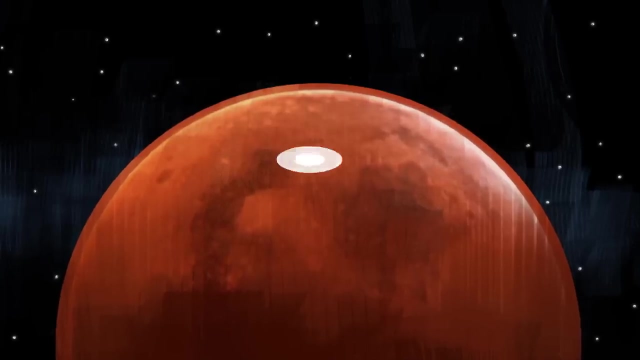 What angle will the probe hit the atmosphere at? What will be the speed of the probe upon entry? Computer simulators run thousands of different landing scenarios, mixing and matching values for all of the variables. Weighing all the possibilities, the computer spits out the potential area of impact. 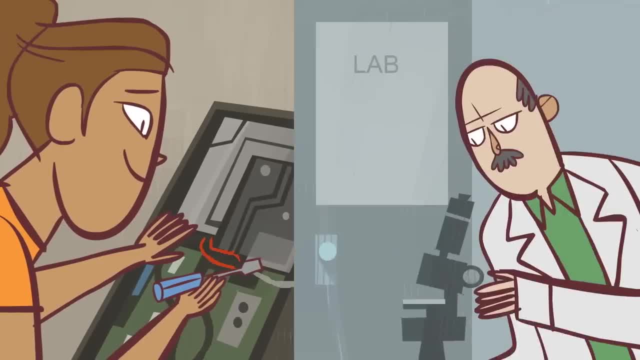 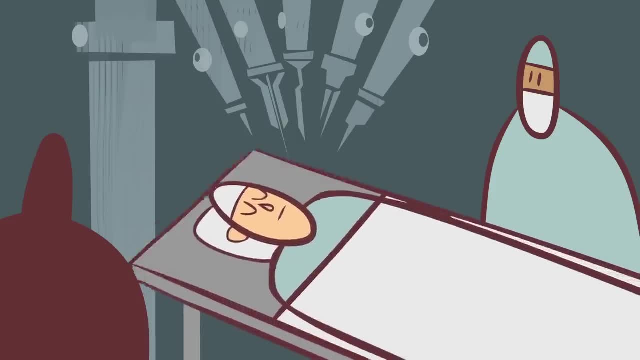 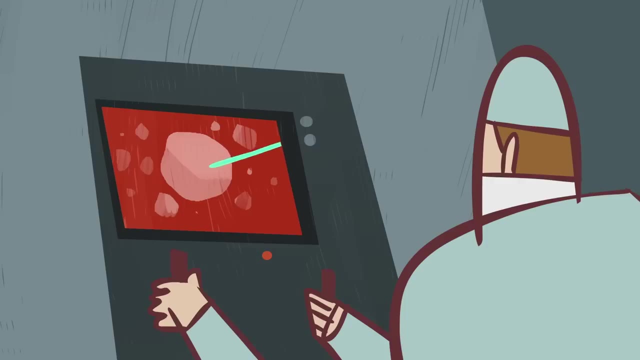 but engineers and researchers often require accuracy on microscopic levels with a high certainty of being right every time. Factories and labs increase precision through better equipment and more detailed procedures. These improvements can be expensive, so managers must decide what the acceptable uncertainty for each project is. 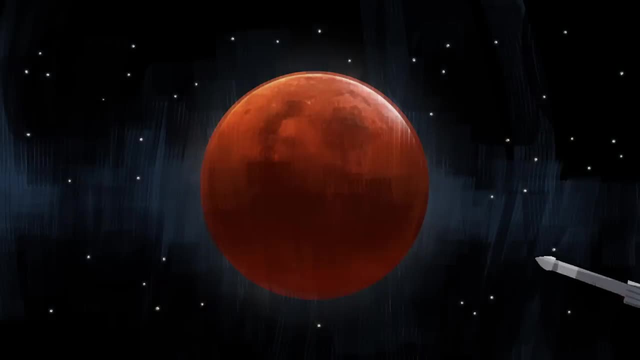 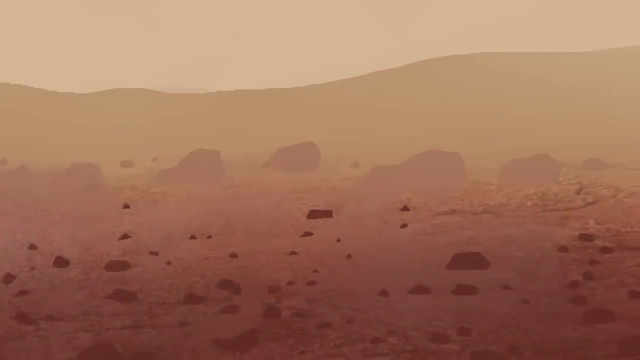 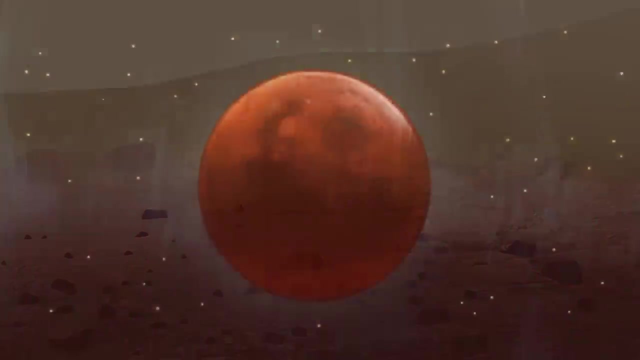 However, investments in precision can take us beyond what was previously possible, even as far as Mars. It may surprise you that NASA does not know exactly where their probes are going to touch down on another planet. Predicting where they will land requires extensive calculations. 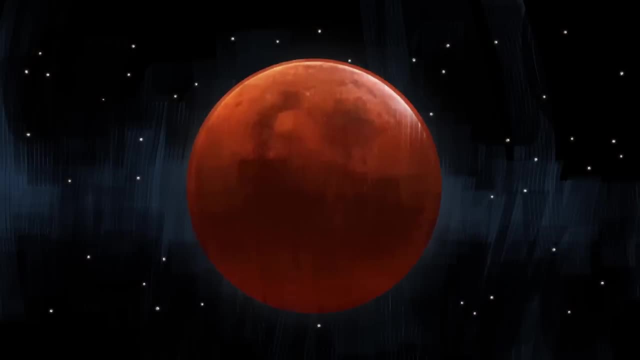 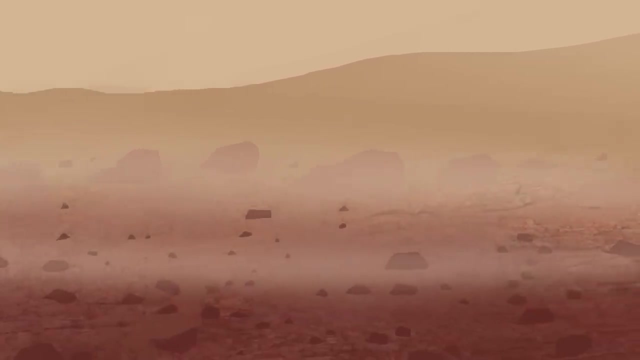 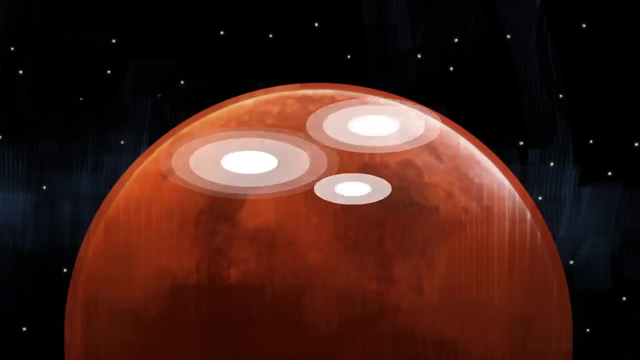 fed by measurements that don't always have a precise answer. How does the Martian atmosphere's density change at different elevations? What angle will the probe hit the atmosphere at? What will be the speed of the probe upon entry? Computer simulators run thousands of different landing scenarios. 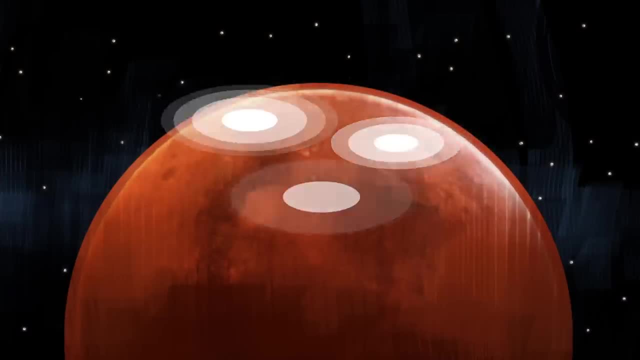 mixing and matching values for all of the variables, Weighing all the possibilities. the computer simulators run thousands of different landing scenarios, mixing and matching values for all of the variables, Weighing all the possibilities. the computer simulators run thousands of different landing scenarios. 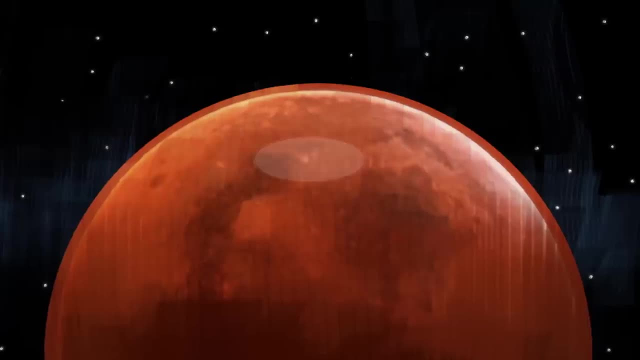 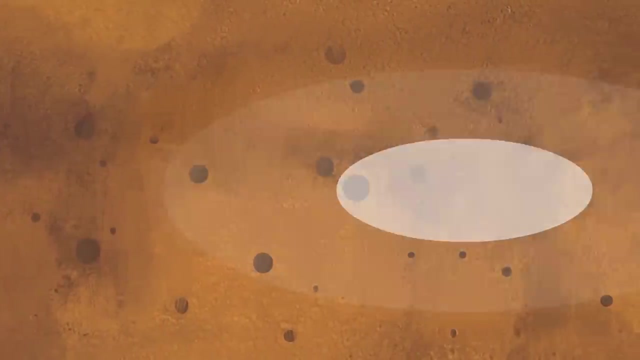 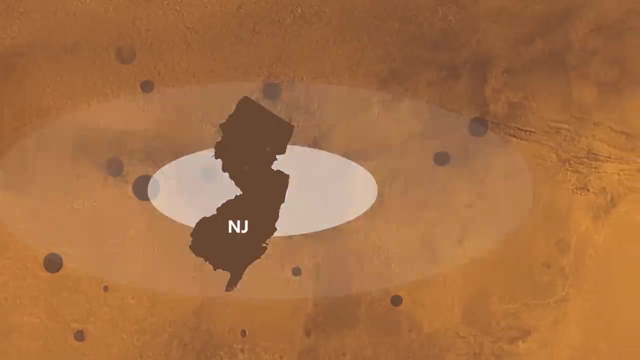 mixing and matching values for all of the variables, The computer spits out the potential area of impact in the form of a landing ellipse. In 1976, the landing ellipse for the Mars Viking lander was 62x174 miles, nearly the area of New Jersey. 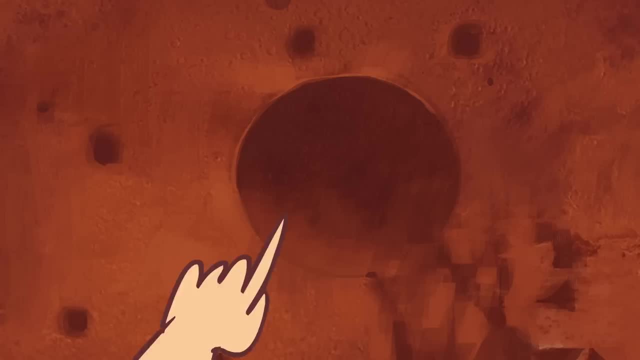 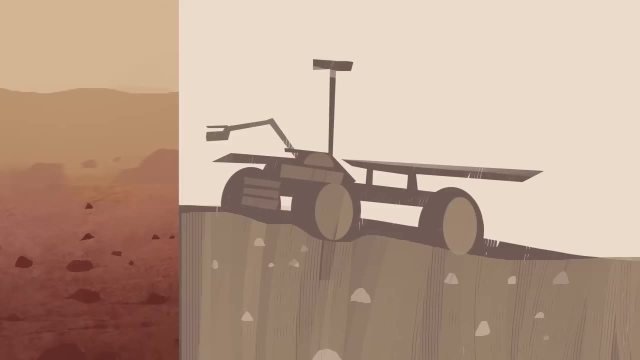 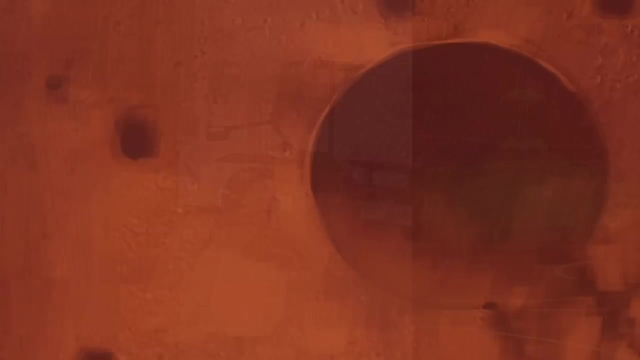 With such a limitation, NASA had to ignore many interesting but risky landing areas. Since then, new information about the Martian atmosphere, improved spacecraft technology and more powerful computer simulations have drastically reduced uncertainty. In 2012,, the landing ellipse for the Curiosity lander. 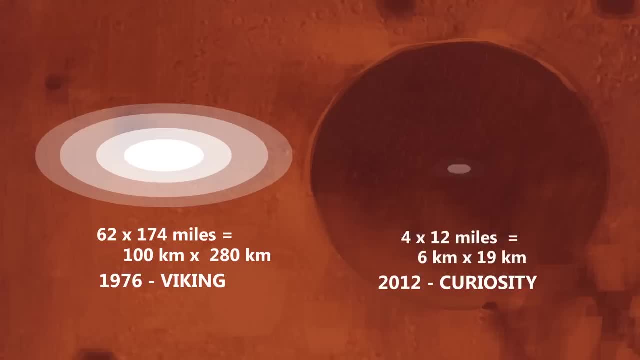 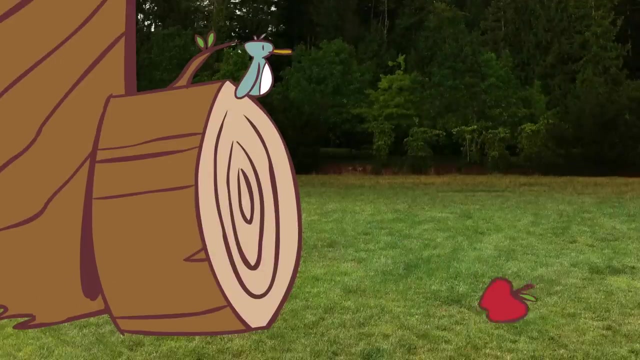 was only 4 miles wide by 12 miles long, an area more than 200 times smaller than Viking's. This allowed NASA to target a specific spot in Gale Crater, a previously unlandable area of high scientific interest. While we ultimately strive for accuracy, 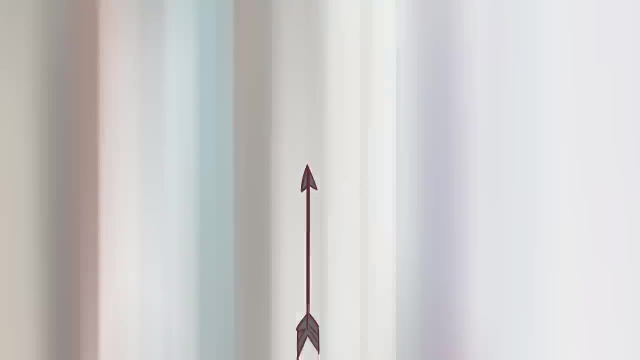 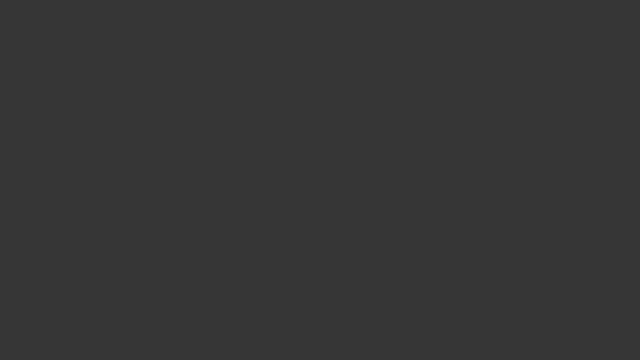 our decision reflects our certainty of reliably achieving it. With these two principles in mind, we can shoot for the stars and be confident of hitting them every time.